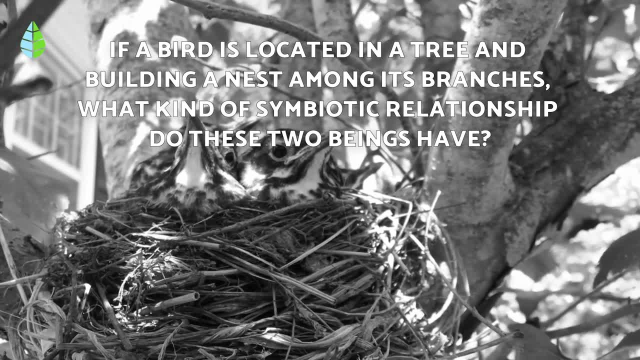 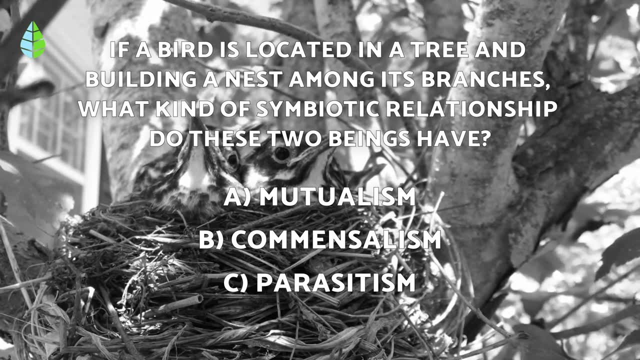 If a bird is located in a tree and building a tree, it will not harm the other. What kind of symbiotic relationships do these two beings have? Is it A Neutralism, B- Commensalism or C- Parasitism? 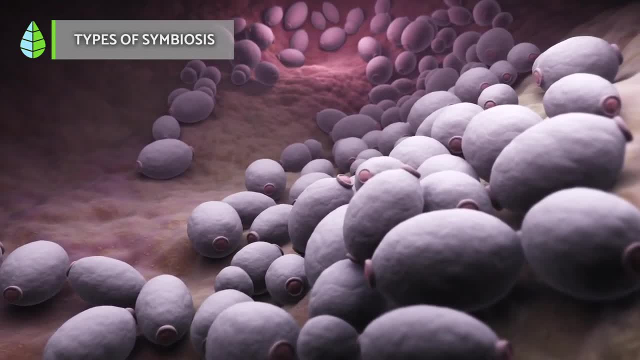 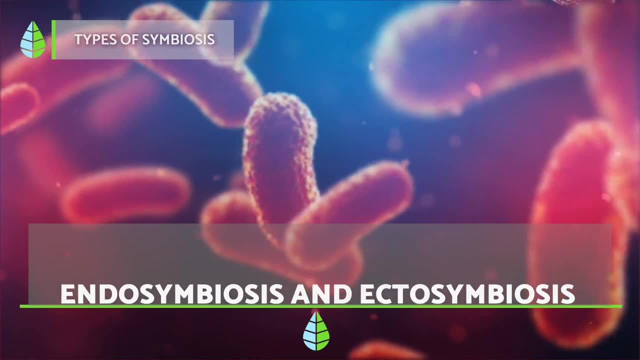 On the other hand, depending on whether one of the symbionts lives inside the other or not, they can be classified into endosymbiosis or ectosymbiosis. It's endosymbiosis if the organism lives inside the cells of the other. 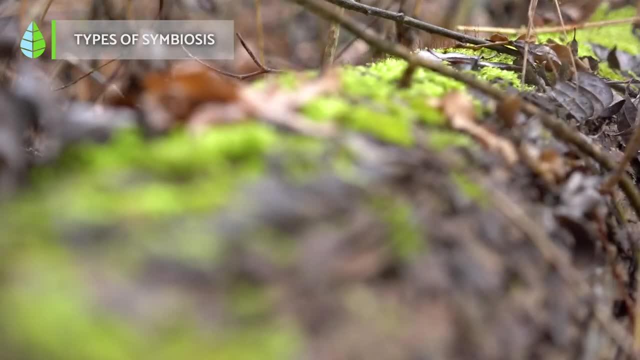 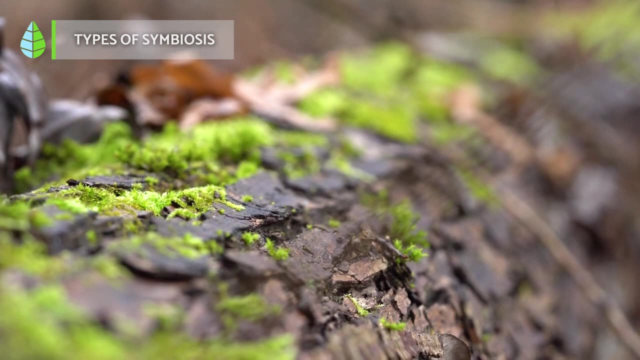 symbiont or in the gaps between them. On the other hand, it is active symbiosis if the symbiont can survive on the outside of the host cells. For example, it can be found on the surface of the digestive tract, exocrine glands or externally on. 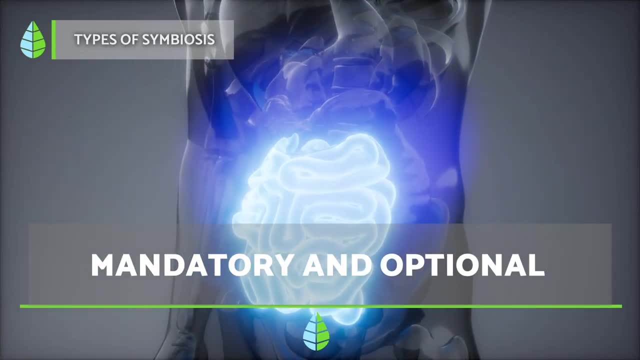 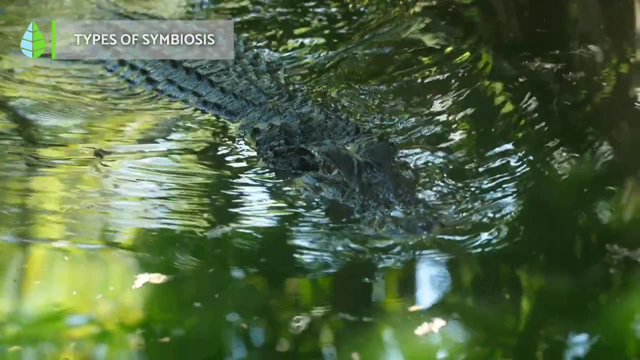 their body. In addition, they can also be classified as mandatory when the relationship is necessary for one of the participants to survive, and optional when the relationship benefits at least one of the organisms but it's not necessary for it to survive. Lastly, depending on the way in which this 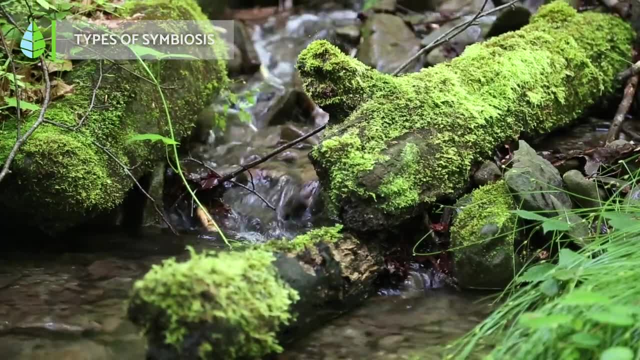 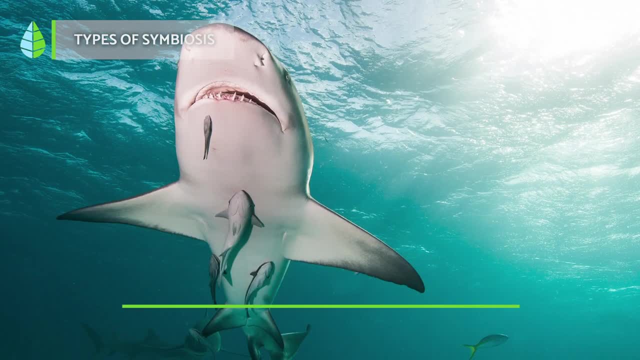 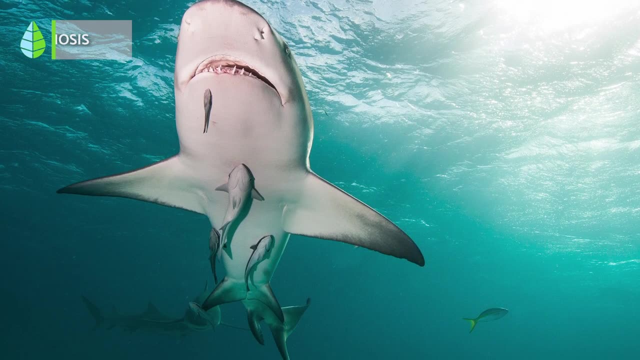 relationship has been established. a distinction can be made between the symbiotic relationships of vertical transmission, when the symbionts are transmitted to the offspring, or the symbiotic relationships of horizontal transmission, when the host organism obtains a symbiont from the environment. generation after generation, Examples of Symbiosis. Here are some examples of: 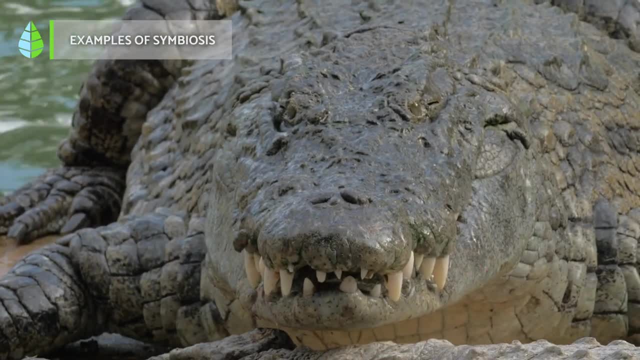 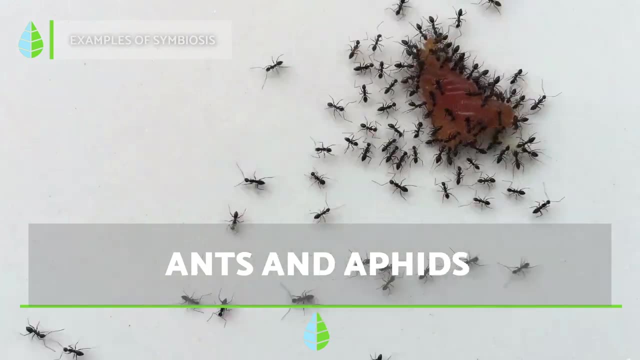 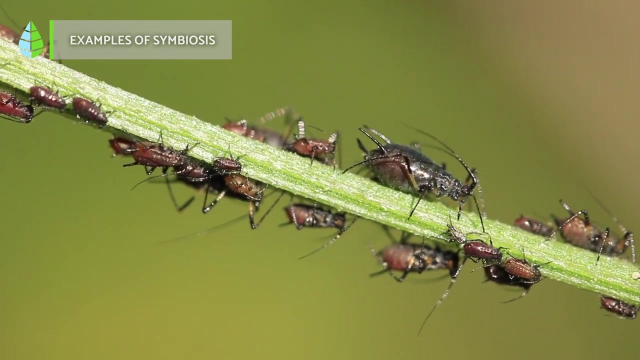 symbiosis, so that you can better understand the importance of these, these types of relationships for the survival of these organisms: Ants and Aphids. Some species of ants, such as the black ant, protect herds of aphids that, in return, provide them with food and honeydew, a sugary substance. 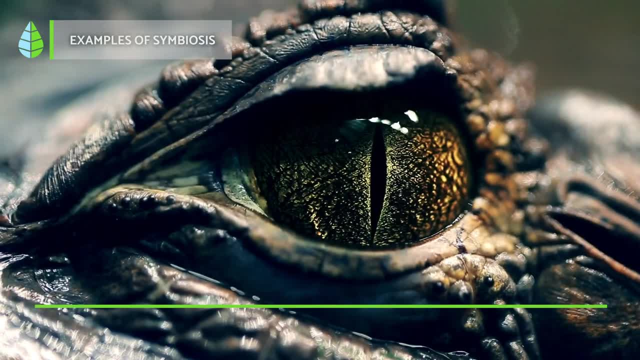 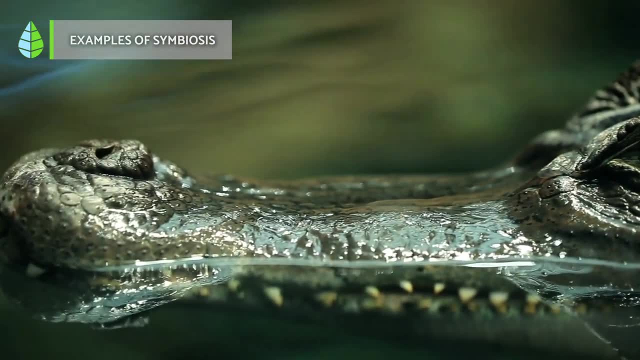 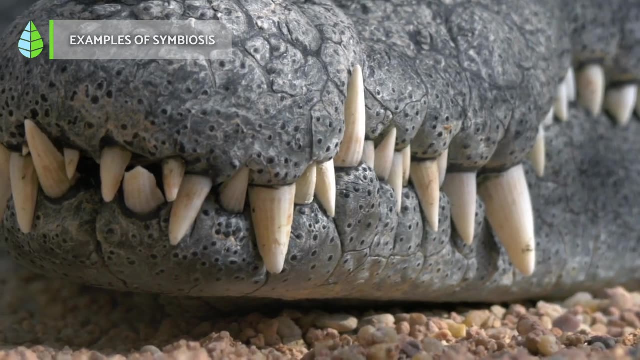 that they produce rich in carbohydrates. Crocodiles and Plovers. We all know the great power that crocodiles have in their jaws. The downside of their aedy teeth is that food debris can cause serious problems such as infections. Thus arises the relationship with the Egyptian plovers, who obtain their food by cleaning.